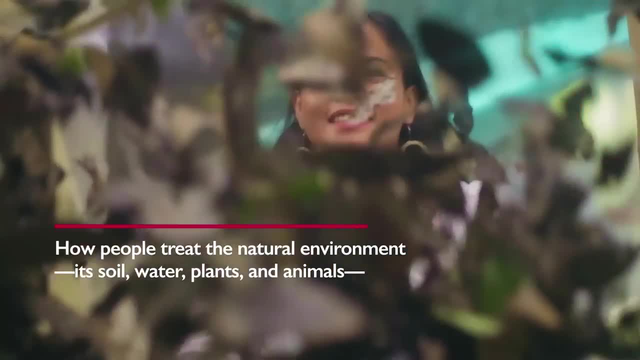 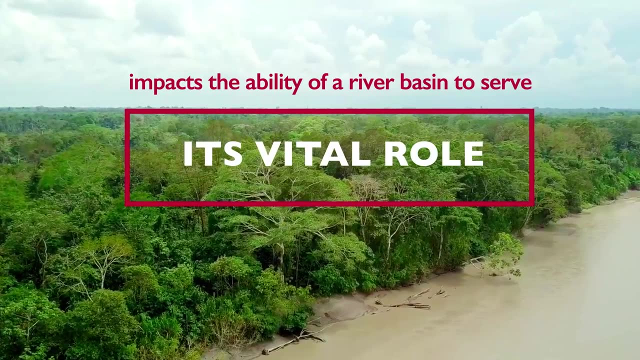 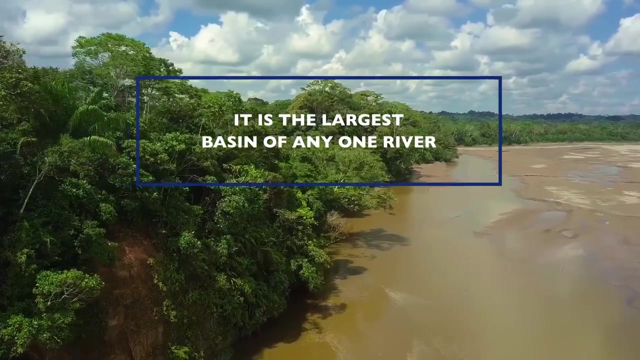 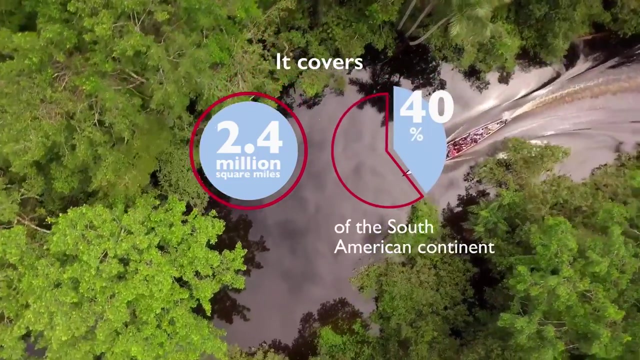 How people treat the natural environment, its soil, water plants and animals impacts the ability of a river basin to serve its vital role. The Amazon river basin is very large. In fact, it is the largest basin of any one river. It covers 2.4 million square miles, or almost 40% of the South American continent. 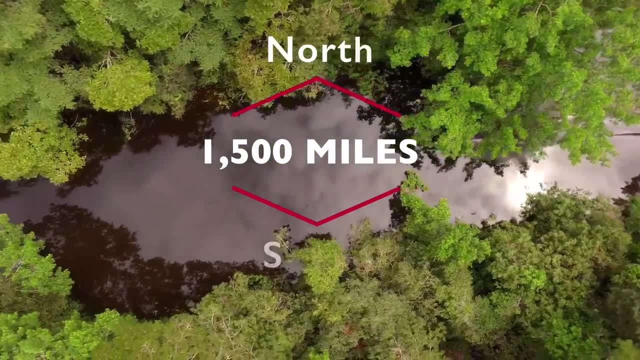 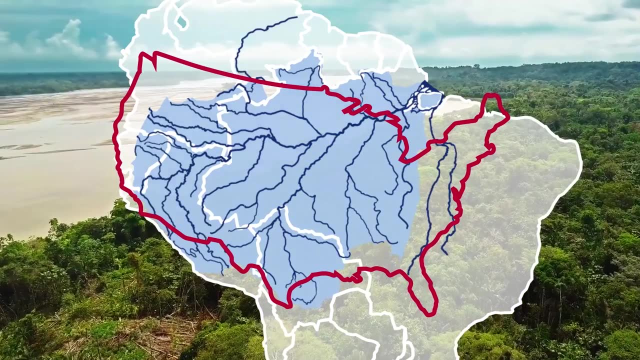 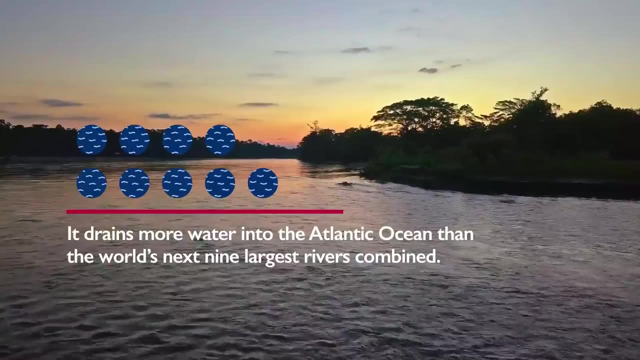 The basin stretches more than 1,500 miles from the ocean From north to south. at its widest point, which is roughly the size of the contiguous United States, It drains more water into the Atlantic Ocean than the world's next nine largest rivers combined. 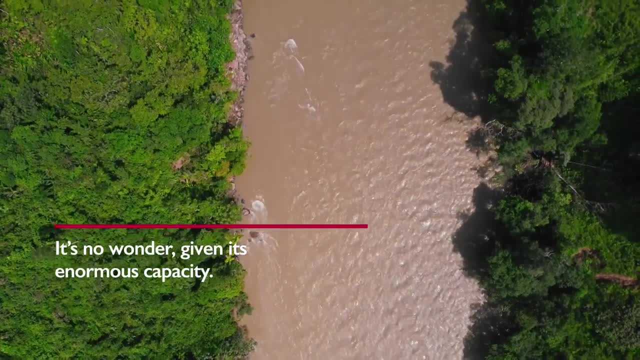 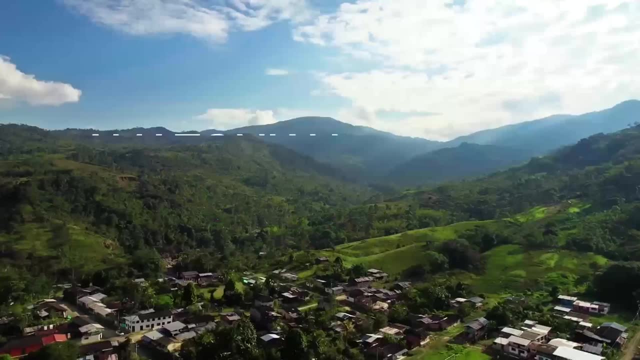 It is no wonder, given its enormous capacity, that the Amazon basin plays a significant role in global carbon and water cycles. More locally, Amazonian communities depend on regular flood cycles within the basin to irrigate and fertilize their agricultural lands, as well as supply the migratory fish that make up a large part of their diets. 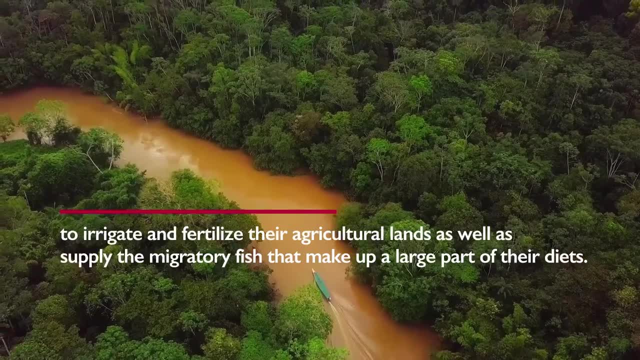 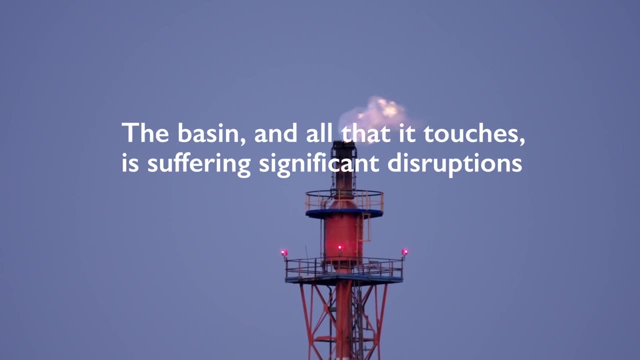 The basin and all that it touches is suffering significant disruptions resulting fromences of other sources of government, else From climate change and illegal activities such as illegal mining and logging Is began objection to the seventeen. For example, climate change is causing flooding in the Western Basin and drought in the Eastern Basin. 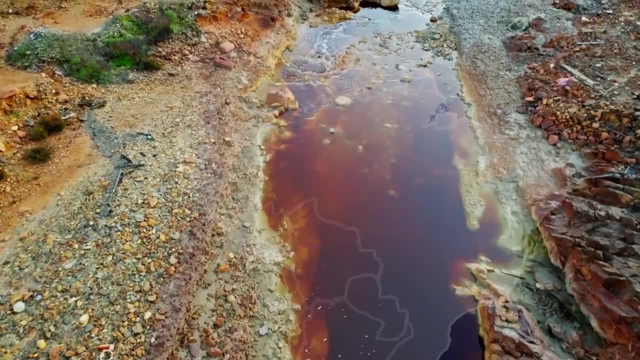 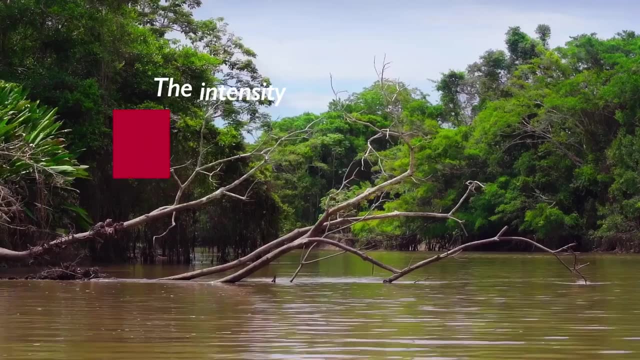 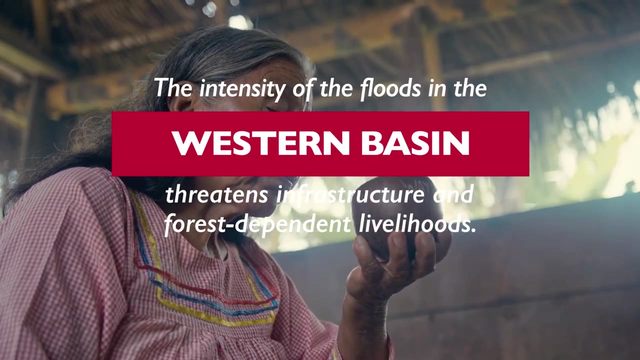 cup60 Ocean. Dest Gill. No One太 hat Tasc sequence. The intensity of the floods in the Western Basin and the� Sea COMMASS A Lots of land. action there, bacteria and biodiversity threatens infrastructure and forest dependent livelihoods In the eastern. 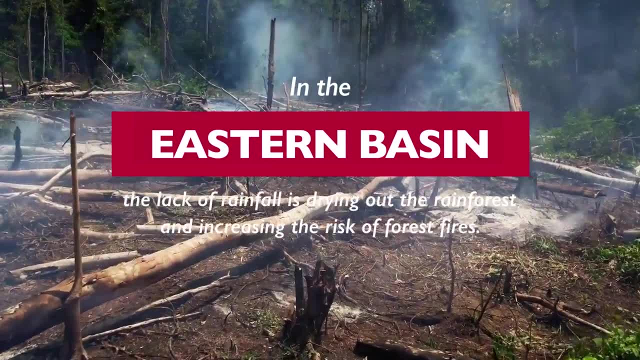 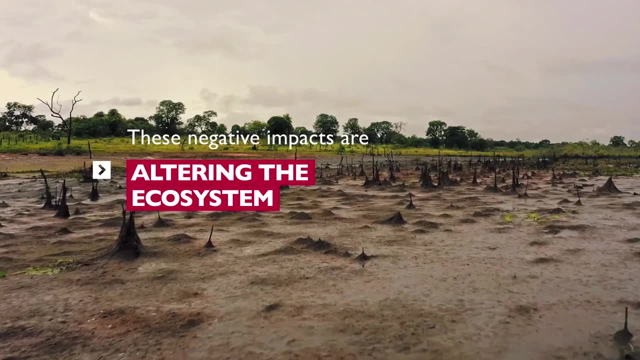 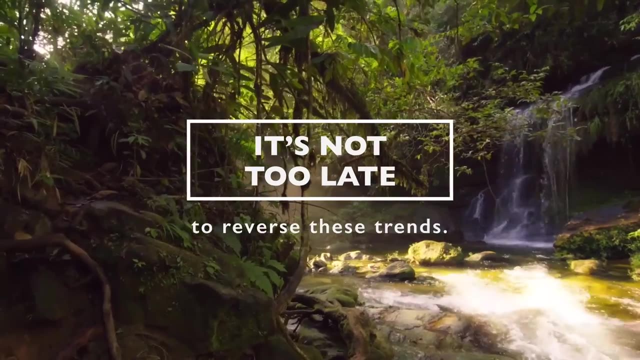 basin. the lack of rainfall is drying out the rainforest and increasing the risk of forest fires. These negative impacts are altering the ecosystem, displacing local peoples and reducing biodiversity. But it's not too late to reverse these trends. The United States Agency for International Development, USAID, through 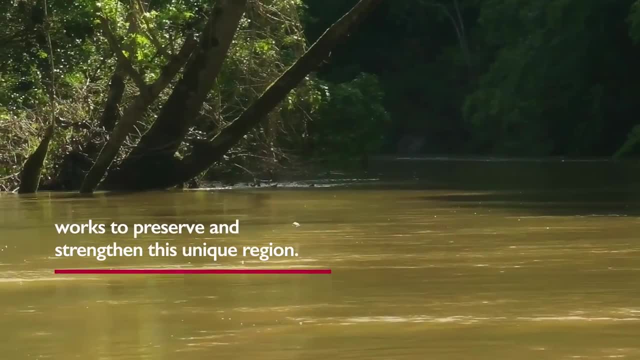 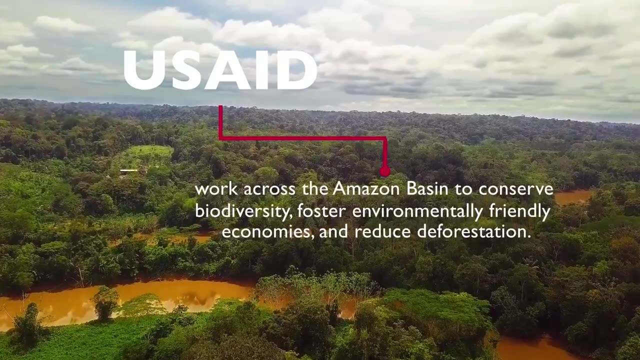 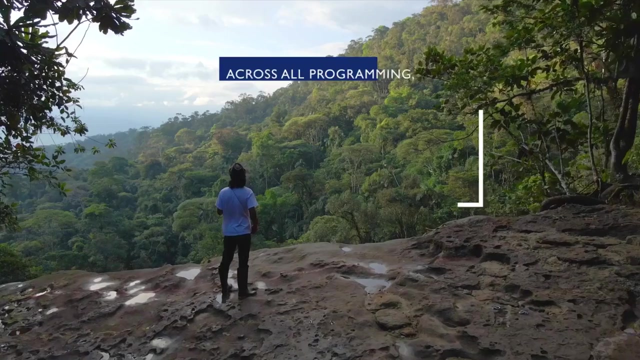 the Amazon Regional Environment Program works to preserve and strengthen this unique region. USAID works across the Amazon Basin to conserve biodiversity, foster environmentally friendly economies and reduce deforestation. Across all programming, USAID works to protect the rights, resources and health of